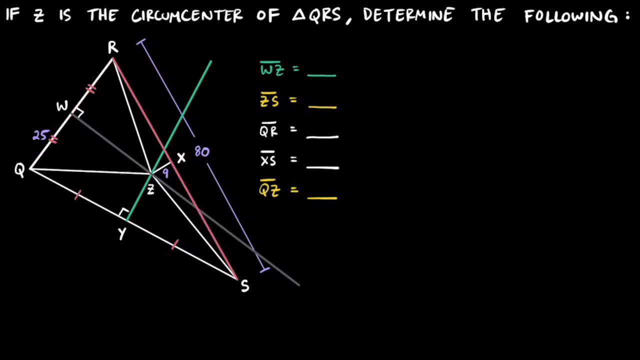 and creates more right triangles. And finally, doing this one more time, with segment RS, if we draw another perpendicular bisector, it creates two congruent segments of RX and XS, And the point where all three of these perpendicular bisectors intersect is called. 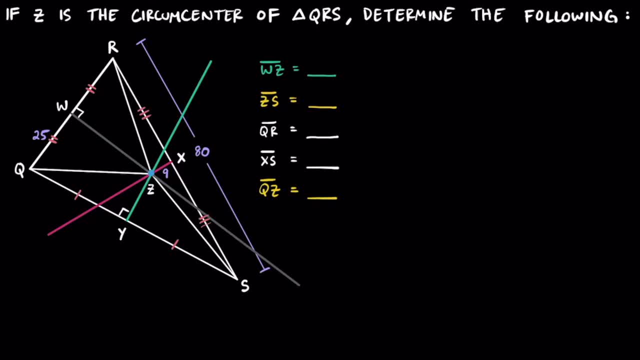 point Z or the circumcenter, Shortening all the perpendicular bisectors. to clean this up a bit, it'll look like this: All three of these perpendicular bisectors intersect and the point where all three of the perpendicular bisectors create right triangles as well as congruent segments. 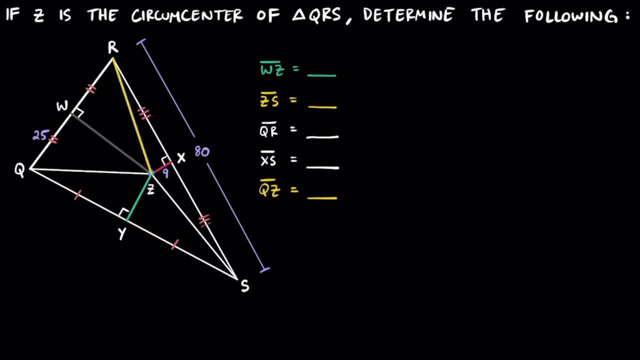 Another unique property that you want to know is that segment RZ, segment QZ and segment SC are all congruent Basically. the distance from the circumcenter to each of the corners or the vertices are all the same. Now let's see if we can use all this information that we know. 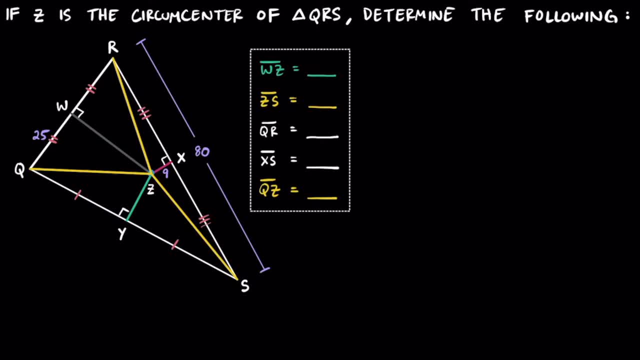 to figure out these five pieces of information. I think one of the easier things to figure out here is going to be finding the length of XS. So if we know that the length of RS is equal to 80,, then the length of XS is going to be 40, because the length of RX is also equal to 40.. 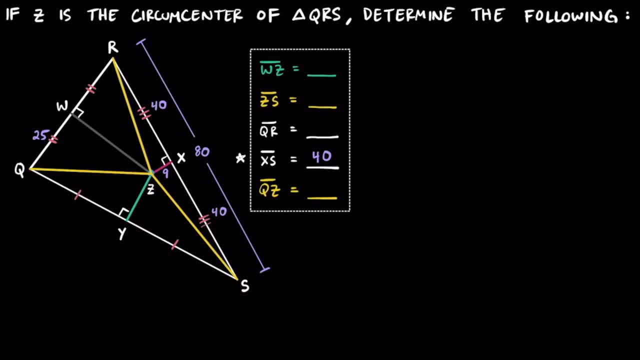 Because we know that point X is the midpoint of segment RS. we know this is going to be true. Another, easier one I think we can do next is figuring out the length of QR. Knowing that the length of QW is equal to 25, that must mean that the length of RW is also equal to 25.. Adding those 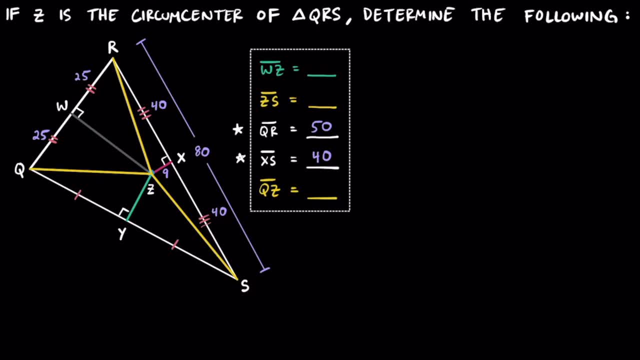 two together, we know the length of QR is going to be equal to 50.. While figuring out those two pieces of information wasn't too bad, the next few are going to take a little bit more work. Let's take a look at segment ZS. Now. looking at segment ZS, I want you to focus in on this. 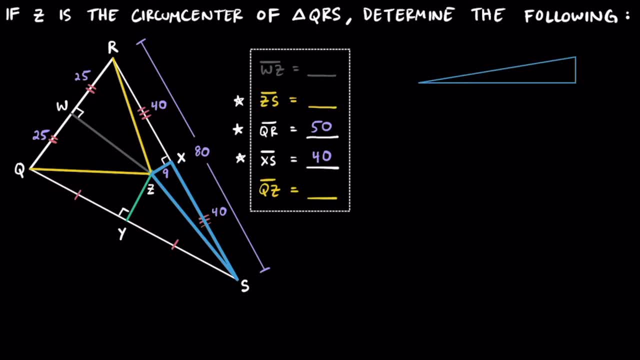 smaller triangle of SXZ. If we rotate that triangle and draw it on the side here, we'd have vertex X over here, S over here and Z up here. Remember, segment XZ represents the perpendicular bisector, so that's where the right angle is. We were given that XZ was equal to 9,. 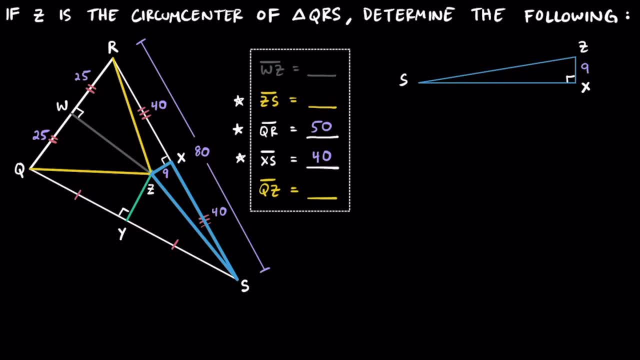 so we can go ahead and label that over here. And we had figured out that segment XZ- represents the xs- was equal to 40.. To find the length of segment zs, we're going to use the legs of these triangles of 9 and 40 to find the length of it, which is the hypotenuse. Remember the two legs or the two? 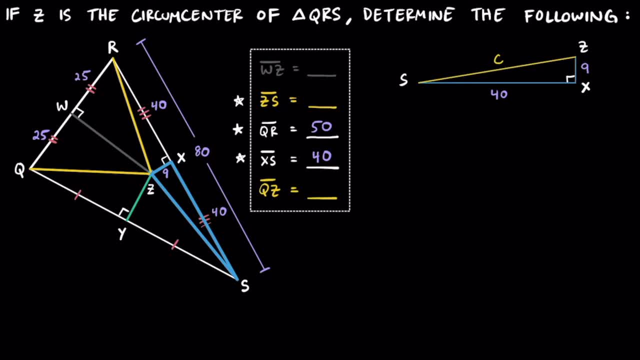 shorter sides of a right triangle always meet at 90 degrees. Writing this out, we would have 40 raised to the second power, plus this 9 raised to the second power, and that's going to be equal to c raised to the second power, or c squared. If we go ahead and square that, 40, 40 times 40,. 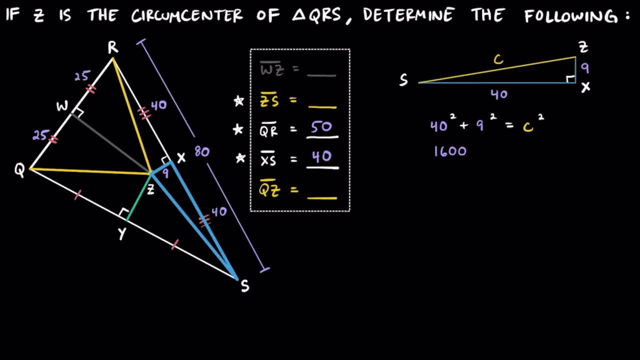 that's going to be 1600, or 1600, and then, if we go ahead and square that 9,, that's going to be 81, so we can go ahead and write 81 here and then c squared. we still don't know. so we're going to. 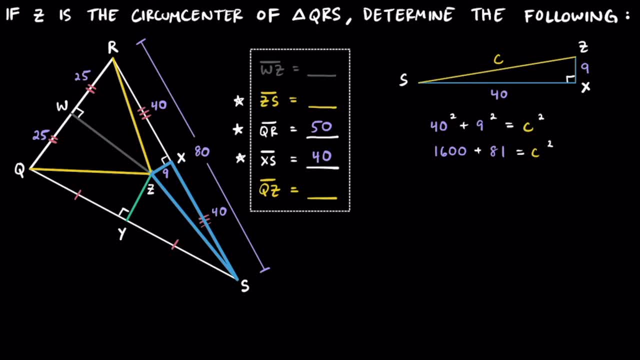 just go ahead and write c squared. If we go ahead and add the 1681,, we're going to get 1681, and that's going to be equal to that c squared again on the other side. and then, if we just go, 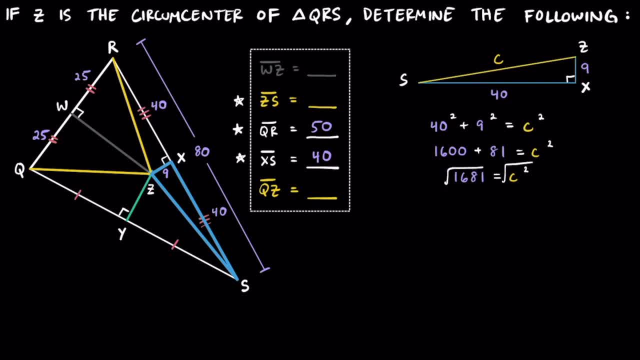 ahead and take the square root from both sides. just like that, we're going to find out that c is going to be equal to 41. And if c is equal to 41, that means segment zs is also equal to 41.. Now, good news for us. 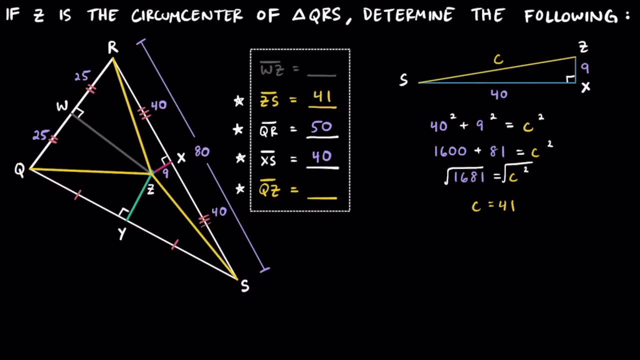 this was actually a bit of a two-for-one deal, because segment qz, remember, is also equidistant from the circumcenter. so if qz is going to be the same as zs, we can also say that this is also 41.. 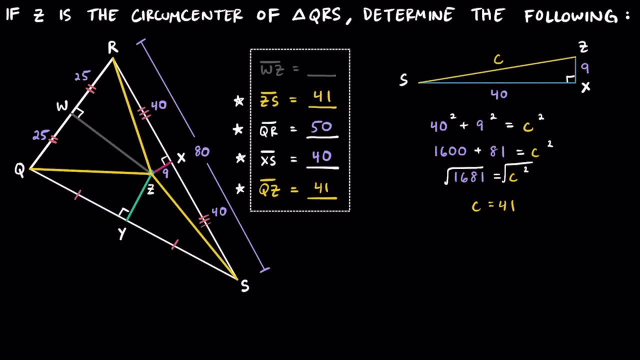 And while we didn't have to find it, segment rz would also be 41.. Finally, let's go ahead and figure out wz. To do that, let's go ahead and focus in on the smaller triangle, of triangle z angle wrz, Rotating it and drawing it to the side. we have vertex w down. here we have r up. 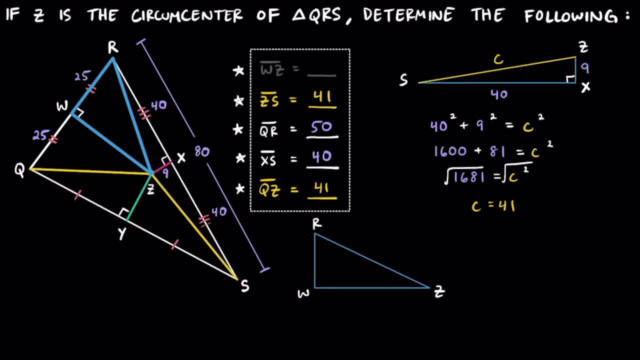 here and then z. Remember segment wz was the perpendicular bisector, so we know that this is going to be the right angle. We also figured earlier that segment wr was equal to 25, and of course rz must be 41, because it's one of those lengths from the vertex to the circumcenter. so it 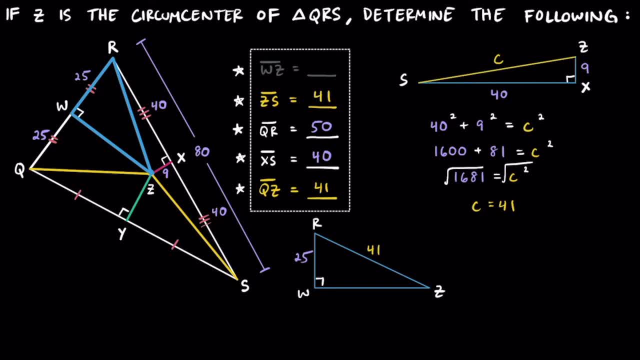 matches the other ones as well. What we have to do is go ahead and figure out the length of wz, Because wz is one of the legs of the circumcenter. we're going to have to figure out the length of the triangle. I'm going to go ahead and call it b. You can call it a2, that's perfectly fine. 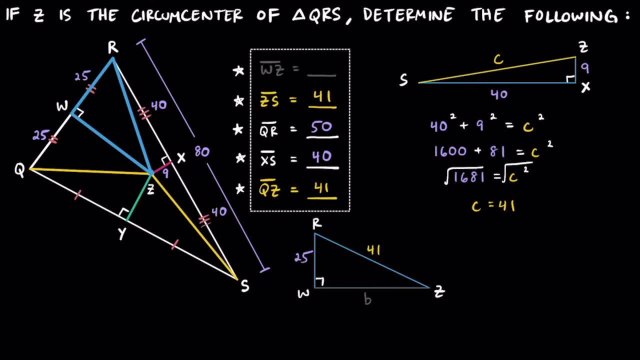 just don't call it c, because it's not the hypotenuse Writing this as an equation. we can go ahead and write 25 raised to the second power plus this b raised to the second power. We don't know what that is. that's what we're looking for And that's going to be equal to. 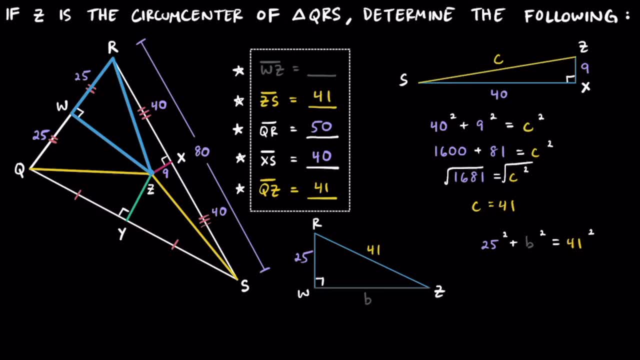 this 41 squared as well. So on the left side, 25 squared, that's going to be 625.. And then we're going to still have this b squared. that is our unknown. And on the other side, let's see what. 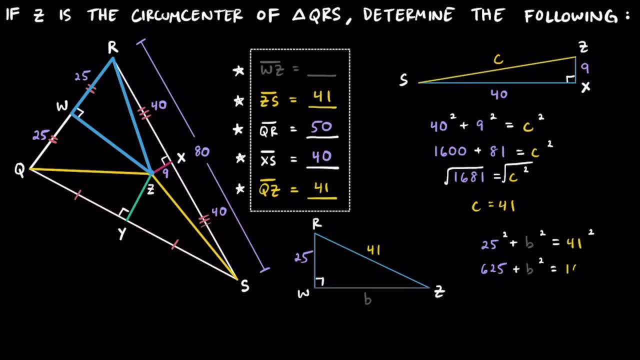 is 41? 41 squared is going to be 1681.. And if we go ahead and subtract 625 from both sides, we're going to be isolating this b, so we have b squared is equal to, and let's see 1681 minus. 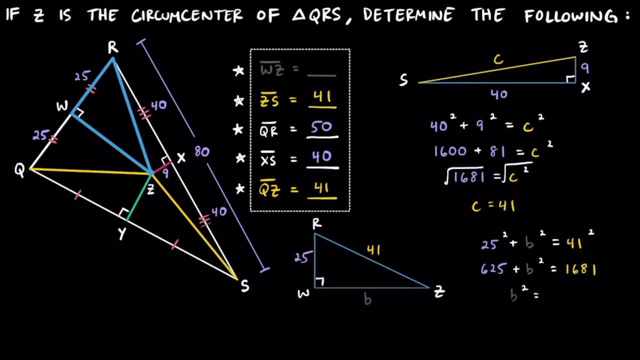 the 625, that's going to equal, I think, 1056.. And then, finally, we go ahead and take the square root of both sides. I don't think 1056 is a perfect square, so we might have to do some work. 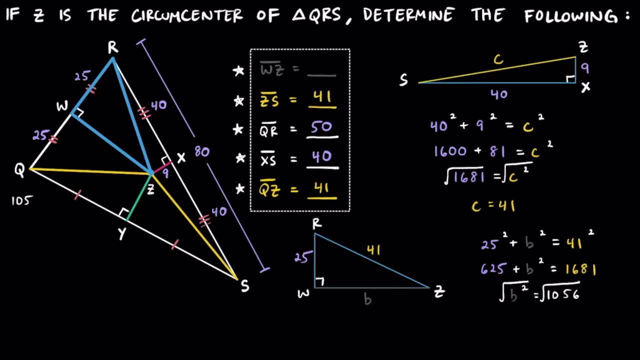 on the side here. So, because 1056 isn't a perfect square, we're going to have to try to simplify the radical a bit here. So let's go ahead and find out what kind of factors we can pull out that are perfect squares. So 2 goes into this, because it's even that's going to be 528.. We're going to put a 2. 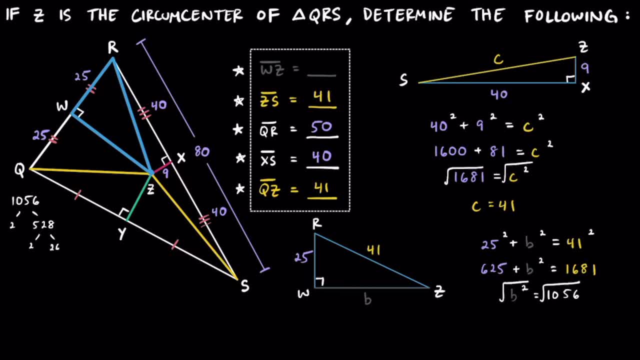 into this one that's going to be 264.. And we put another 2 into this that's going to be 132.. Another 2 into this: that's going to be 66.. And another, let's put a 3 into it this time. 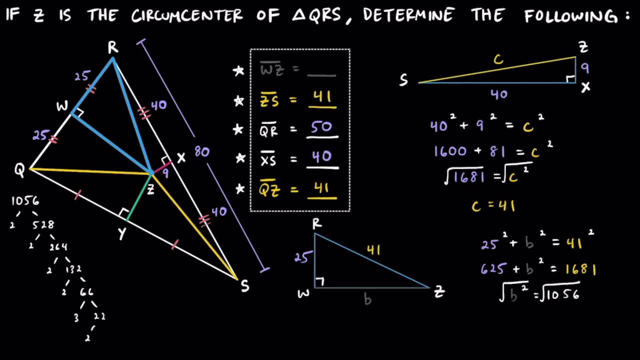 that's going to be 168.. And then we're going to put another 2 into this. that's going to be 168.. That's going to be what? 22.. Oh, and one more 2, so that's going to be 11.. So any pair of common? 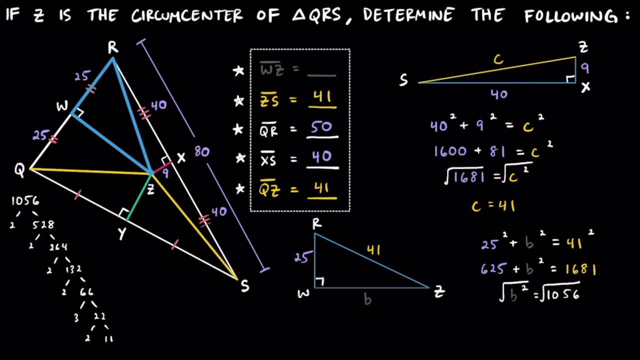 primes is going to make a perfect square, so that's going to be helpful to us. So this 2 and 2 here make 4, that's a perfect square, so that's going to be part of something we can pull out. Another: 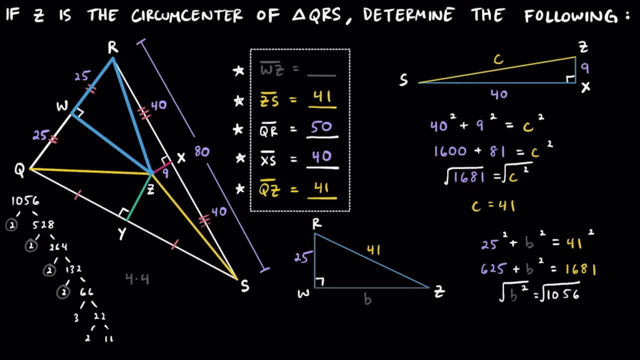 2 and a 2 together make another 4, that's another perfect square, And I think that's it. So 4 times 4 is 16, and then so we have 16 as part of this, so we'll have 16.. 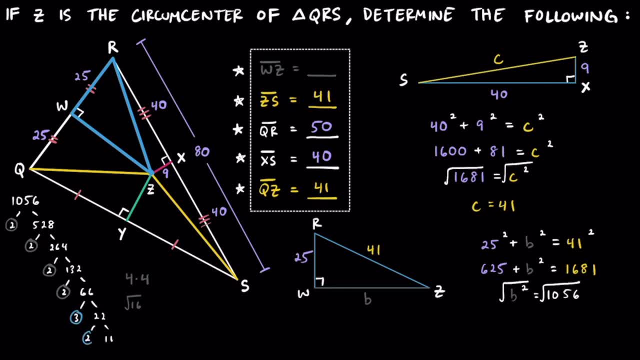 And then what wasn't a perfect square? Well, this didn't have a partner, this didn't have a partner and this didn't have a partner. So put that all together and that's going to be root 66.. So it turns out that 16 times 66 is equal to that 1056.. But what's nice about the root 16 is